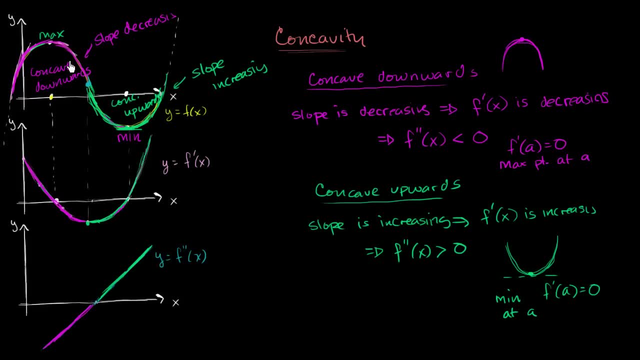 But we see here that there's a point at which we transition from being concave downwards to concave upwards. Before that point, the slope was decreasing And then the slope starts increasing. The slope was decreasing And then the slope started increasing. 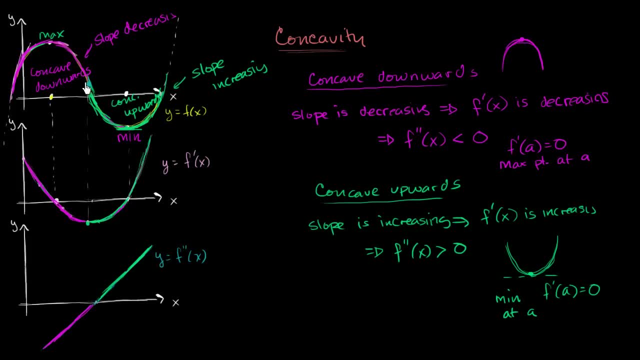 So that's one way to look at it. Right here in our function, we go from being concave downwards to concave upwards. When you look at our derivative, at that point, our derivative went from decreasing to increasing. And when you look at our second derivative, at that point, 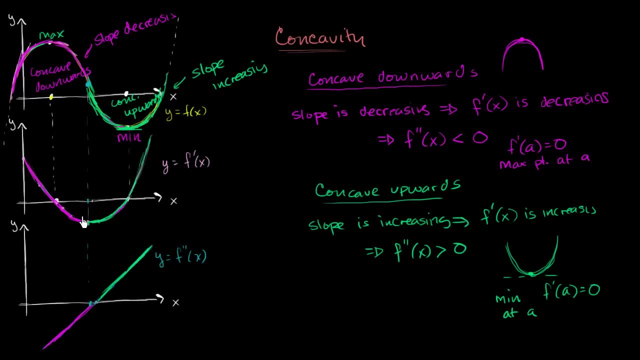 it went from being negative to positive. So this must have some type of a special name. you're probably thinking- And you would be thinking correctly- This point at which we transition from being concave downwards to concave upwards, or the point at which our derivative has 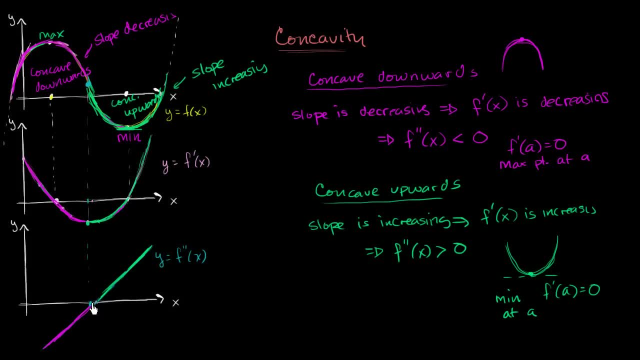 an extremum point, or the point at which our second derivative switches signs like this. we call it an inflection point, And the most typical way that people think about how could you test for an inflection point? it's a point. Well, conceptually, it's where you go from being a downward 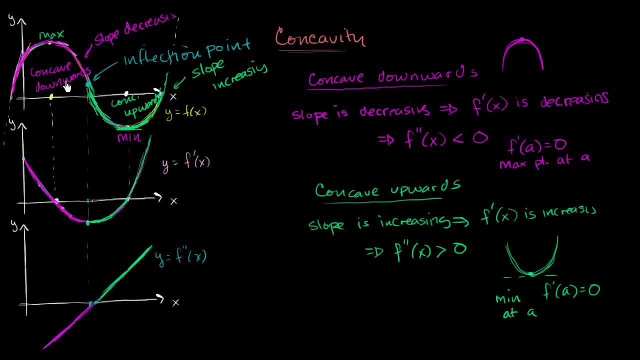 opening u to an upward opening u, or when you go from being concave downwards to concave upwards. But the easiest test is: it's a point at which your second derivative switches signs. So in this case, we went from negative to positive. 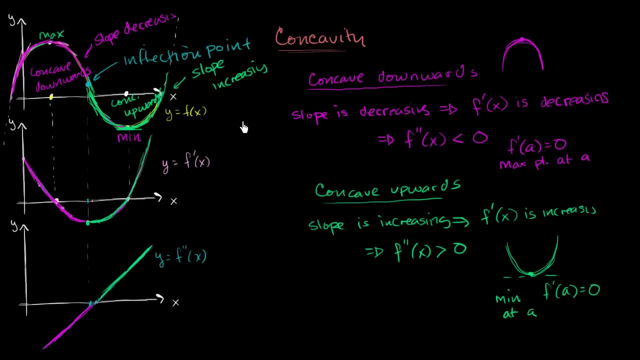 But we could have also switched from being positive to negative. So inflection point, your second derivative f prime, prime of x switches signs goes from being positive to negative or negative to positive switches signs. So this is a case where we went from concave downwards. 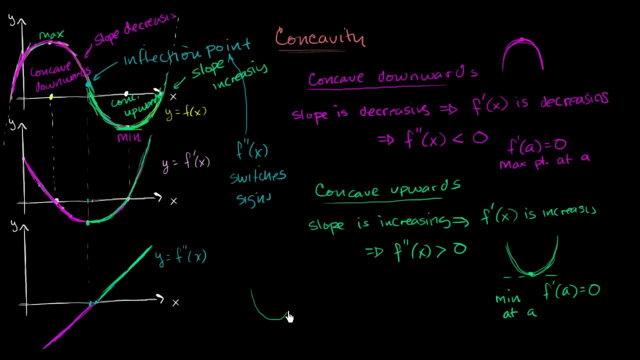 to concave upwards. If we went from concave upwards to concave downwards, like that, then this inflection point, at this inflection point, up until that point the slope was increasing, So the second derivative would be positive, And then the slope is decreasing. 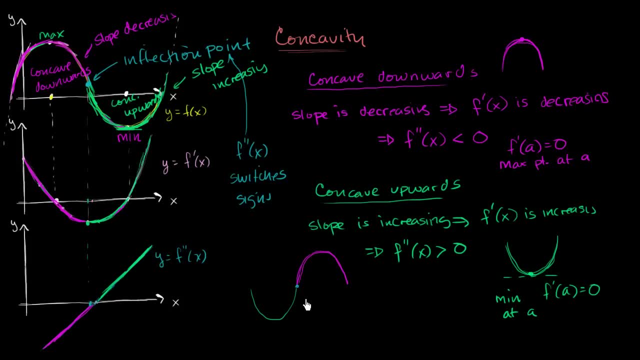 The derivative is decreasing, So your second derivative would be negative. So here your second derivative is going from positive to negative. Here, your second derivative is going from negative to positive In either case. In either case, you are talking about an inflection point.